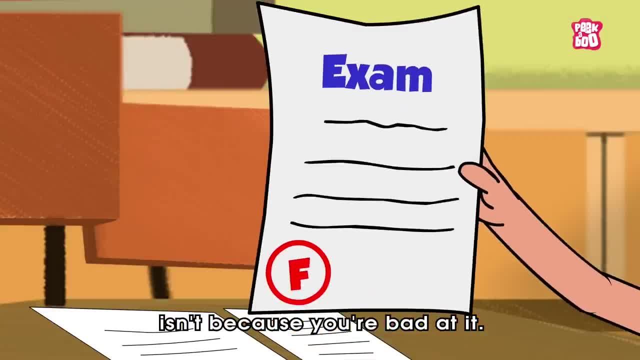 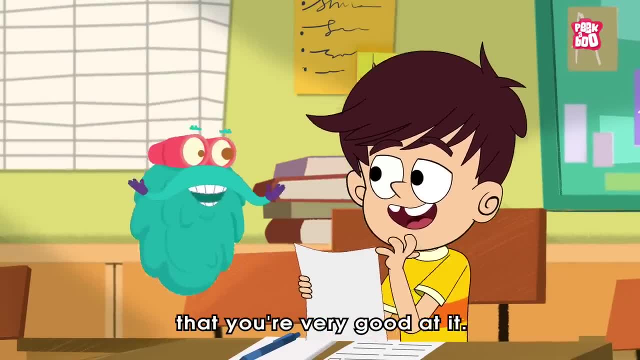 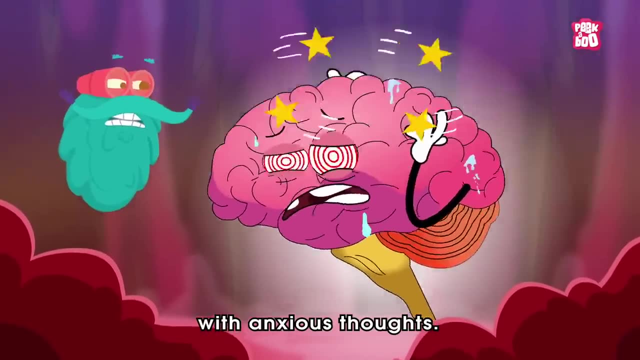 The reason you can't solve math problems isn't because you are bad at it. In fact, there's a fair chance that you are very good at it, But you can't perform because your brain is all jumbled up with anxious thoughts, Confused. 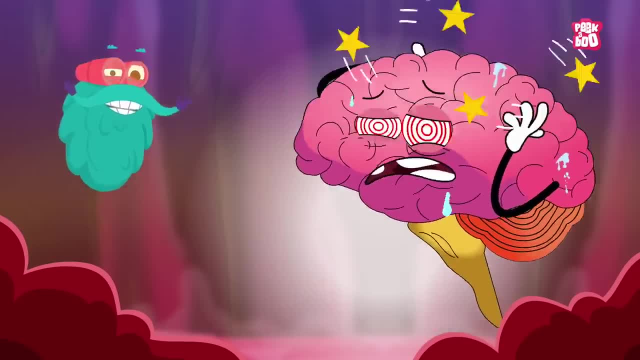 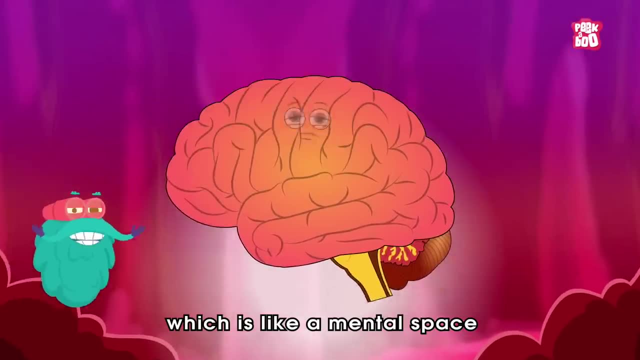 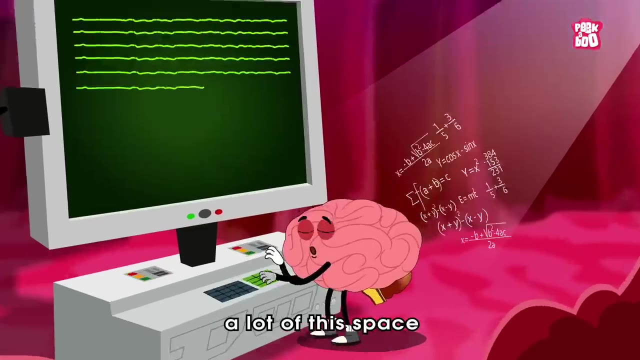 Let me explain it with the help of some science. You see, our brains have something called working memory, which is like a mental space where we solve problems When we're doing math, a lot of this space should be used for solving math problems. 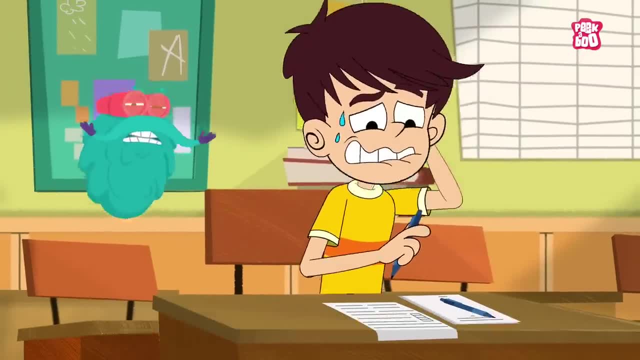 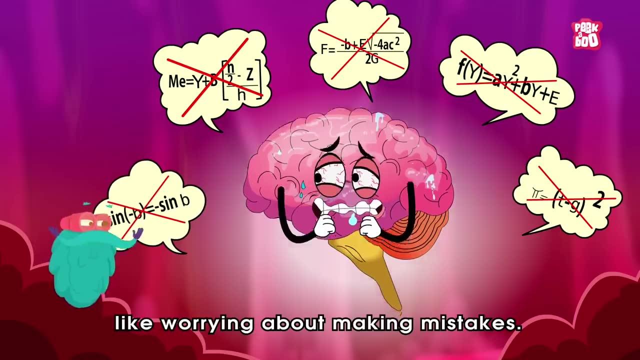 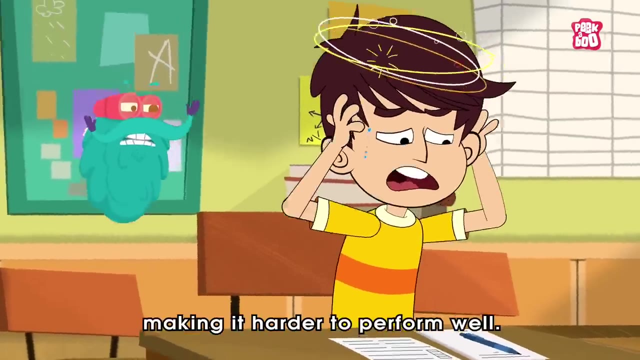 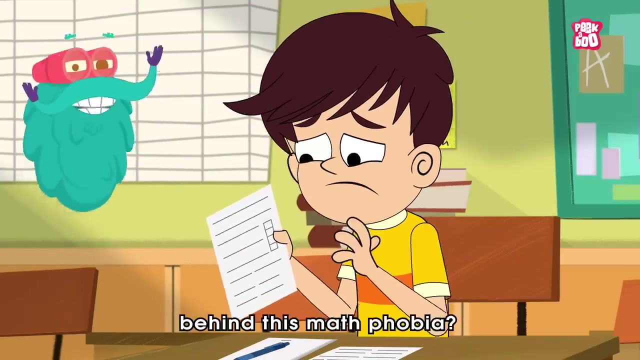 But when someone has math anxiety, a significant part of that space is taken up by anxious thoughts like worrying about making mistakes. This leaves less room for solving the actual math problems, making it harder to perform well. But what's the reason behind this math phobia? 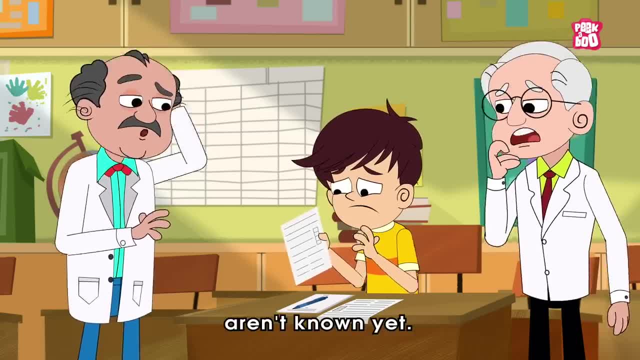 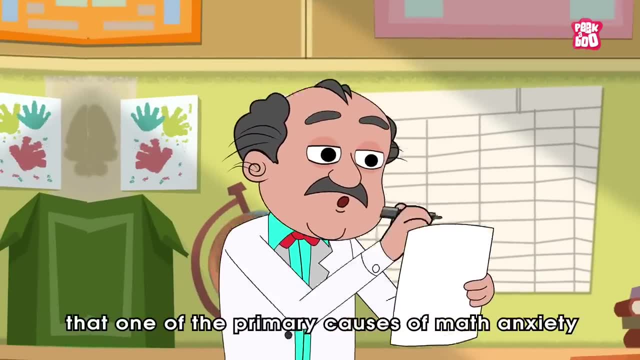 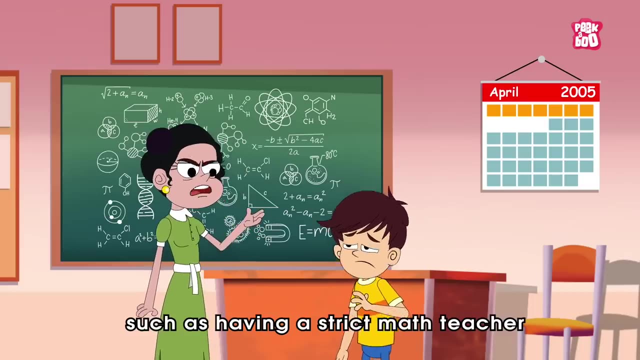 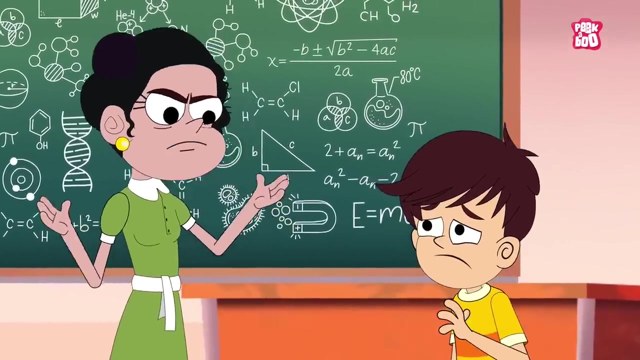 Well, the exact reasons behind it aren't known yet. However, some studies show that one of the primary causes of math anxiety can be attributed to past negative experiences, such as having a strict math teacher who often speaks negatively about your mathematical performance. Furthermore, research has shown that a parent's perception of mathematics 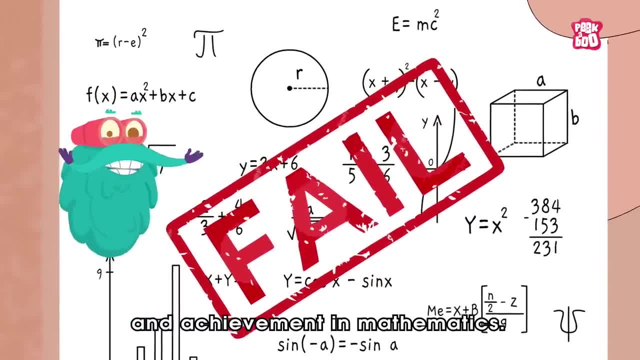 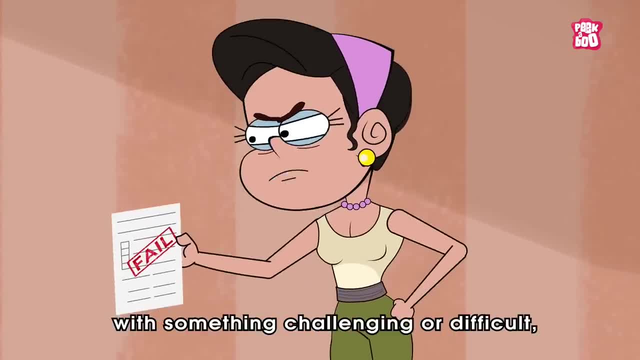 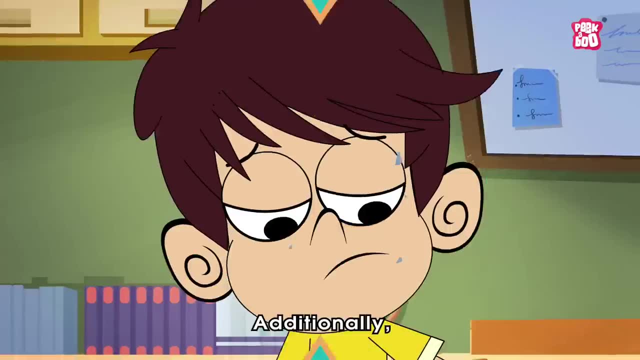 influences their child's perception and achievement in mathematics. If a parent associates math with something challenging or difficult, the child may internalize this message and also find the subject challenging. Additionally, math anxiety can worsen over time due to factors like high-pressure tests. 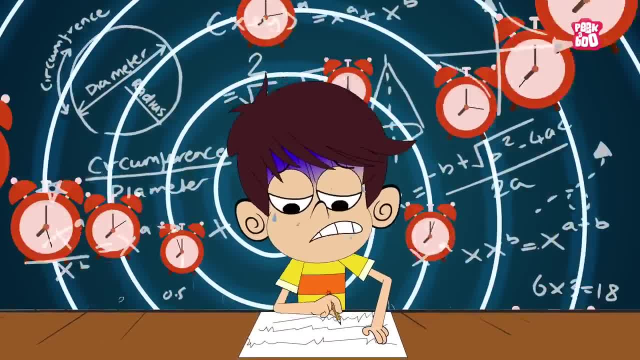 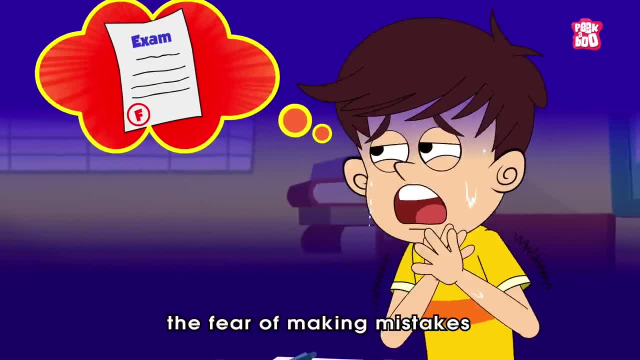 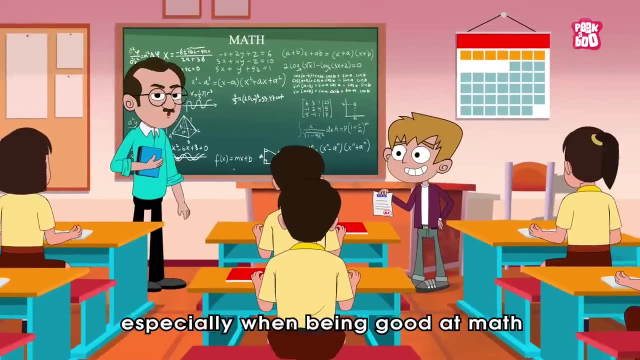 Imagine having to solve a tricky math problem with a timer ticking away That can make anyone anxious. At the same time, the fear of making mistakes or failing math exams can also heighten stress levels, especially when being good at math is considered a sign of smartness in some cultures. 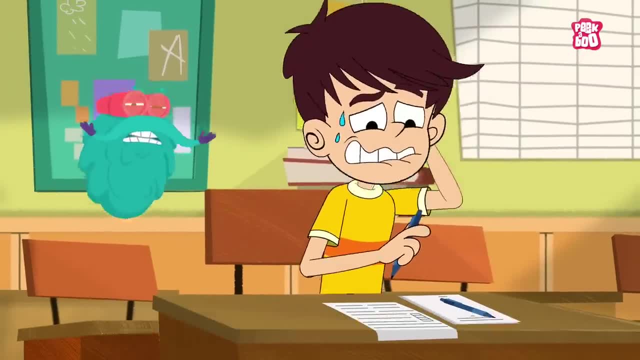 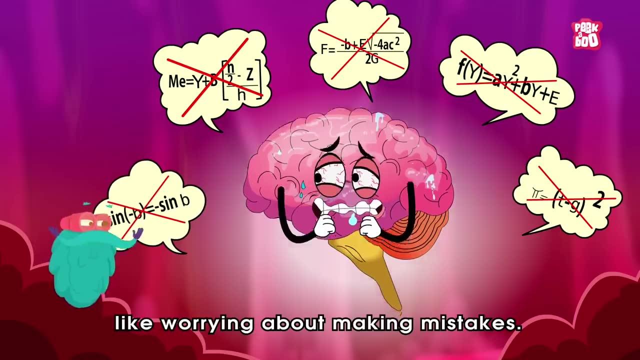 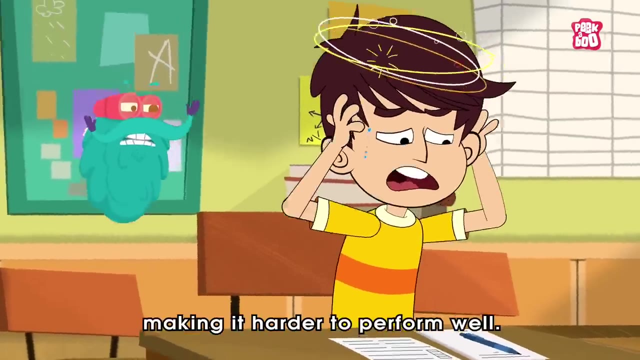 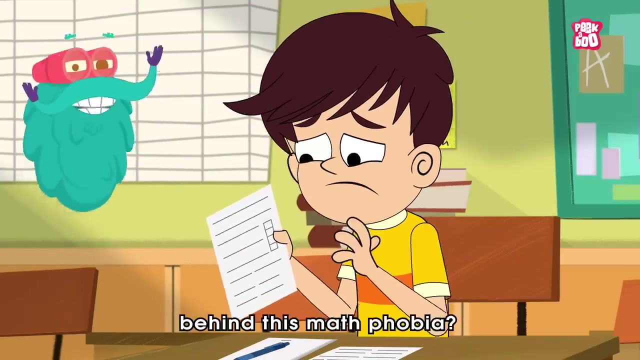 But when someone has math anxiety, a significant part of that space is taken up by anxious thoughts like worrying about making mistakes. This leaves less room for solving the actual math problems, making it harder to perform well. But what's the reason behind this math phobia? 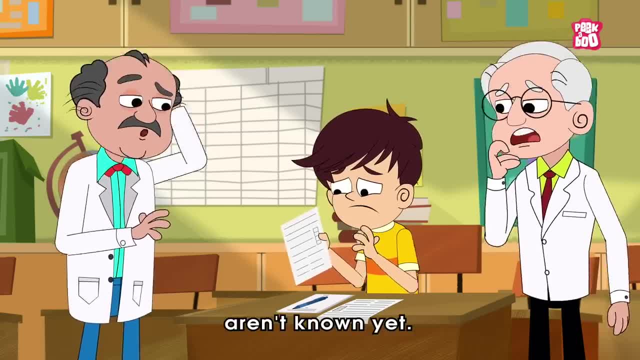 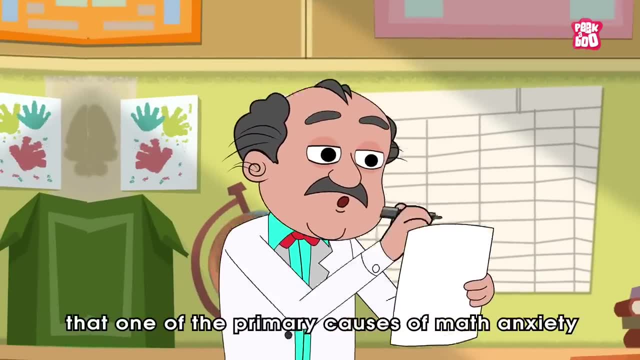 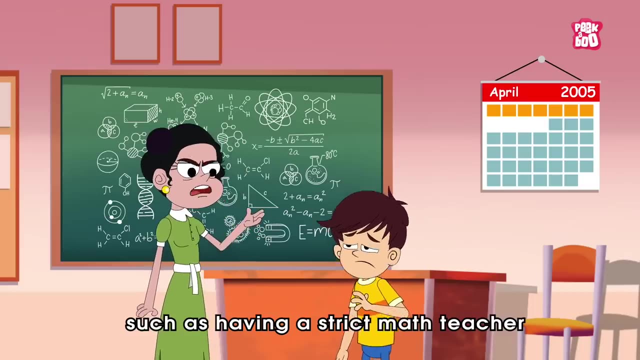 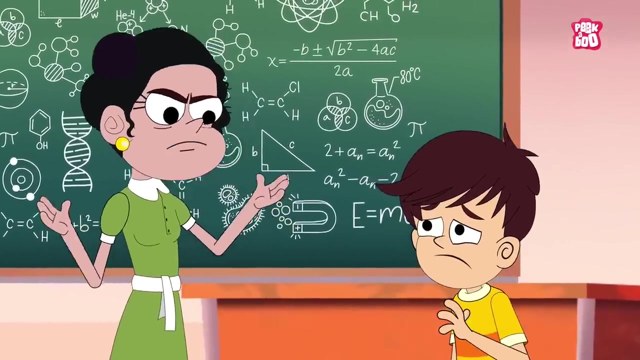 Well, the exact reasons behind it aren't known yet. However, some studies show that one of the primary causes of math anxiety can be attributed to past negative experiences, such as having a strict math teacher who often speaks negatively about your mathematical performance. Furthermore, research has shown that a parent's perception of mathematics 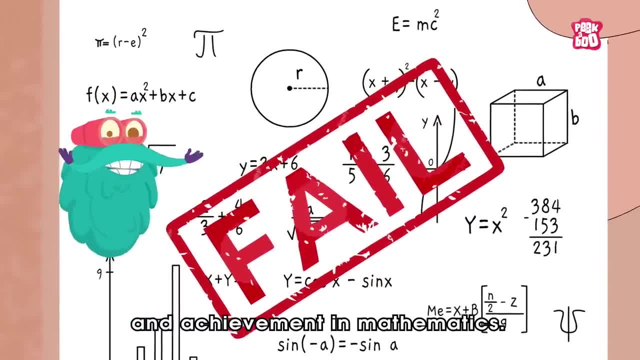 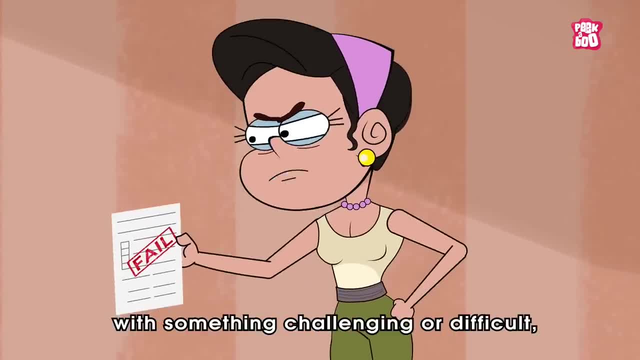 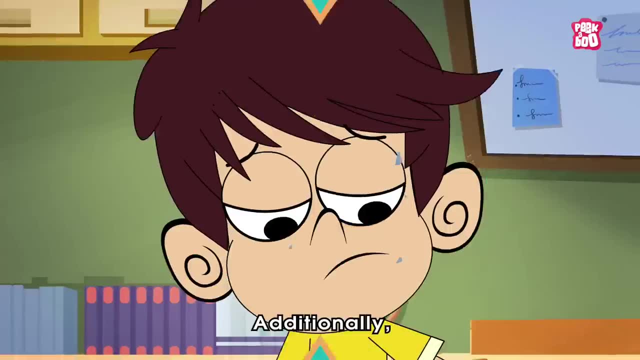 influences their child's perception and achievement in mathematics. If a parent associates math with something challenging or difficult, the child may internalize this message and also find the subject challenging. Additionally, math anxiety can worsen over time due to factors like high-pressure tests. 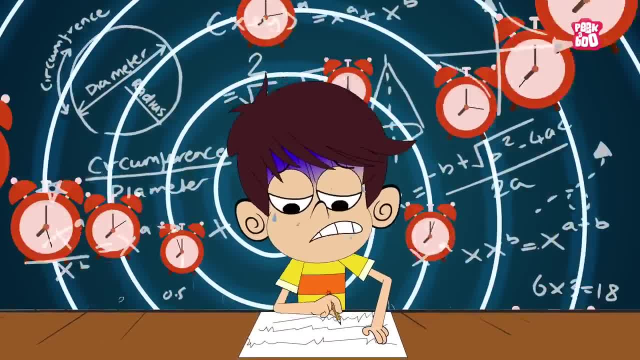 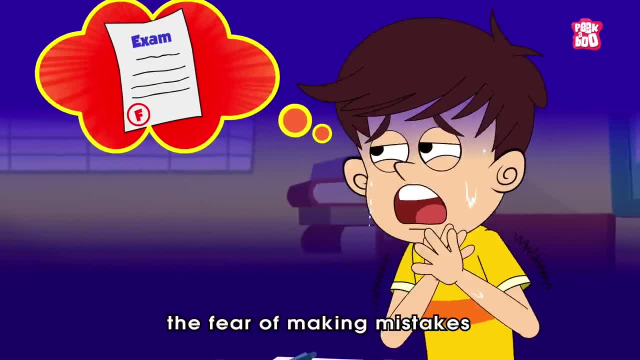 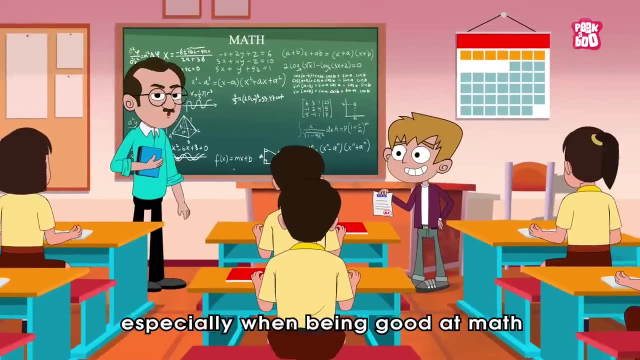 Imagine having to solve a tricky math problem with a timer ticking away That can make anyone anxious. At the same time, the fear of making mistakes or failing math exams can also heighten stress levels, especially when being good at math is considered a sign of smartness in some cultures. 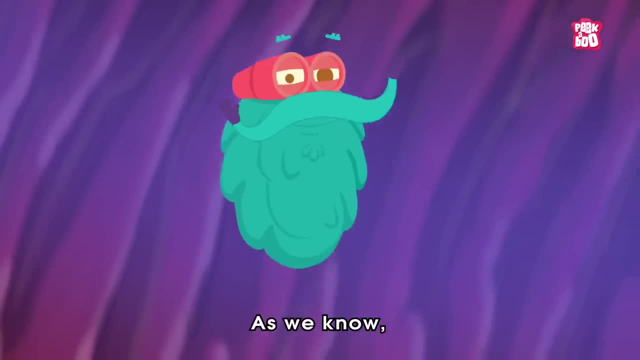 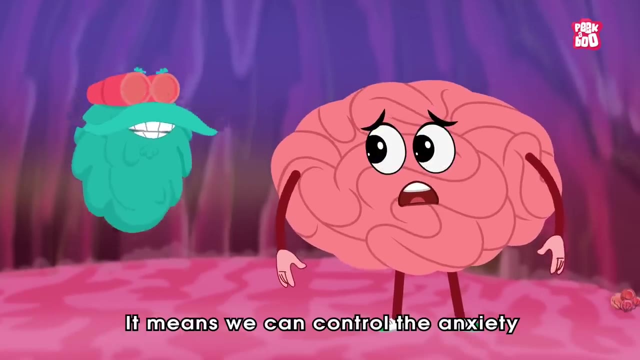 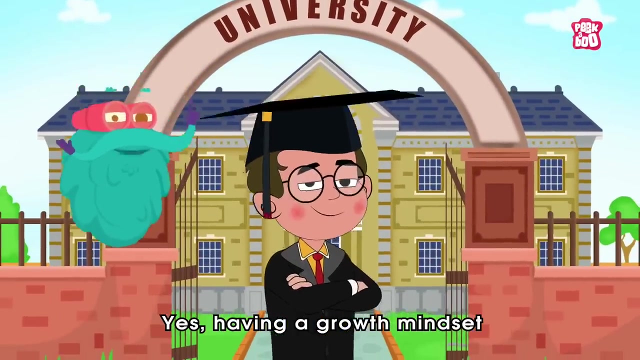 But here's the good news. As we know, math anxiety has more to do with our brains. It means we can control the anxiety by changing our mindset towards math. Yes, having a growth mindset that you can achieve anything can actually help you get better at math. 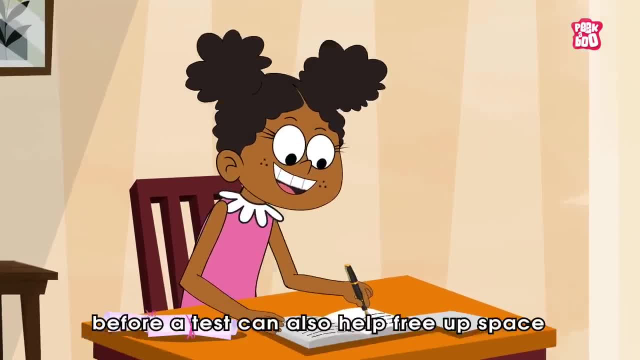 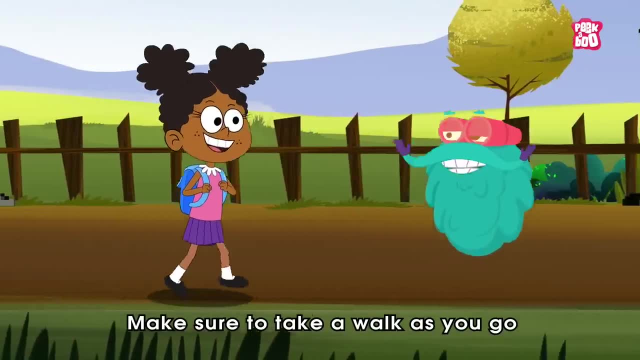 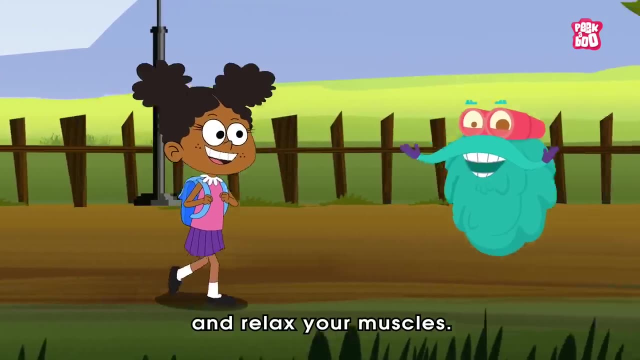 Besides writing down your anxious thoughts before a test can also help free up space in working memory. Make sure to take a walk as you go to attend the test to ease up the tension and relax your muscles, Additionally practicing relaxation techniques such as deep breathing. 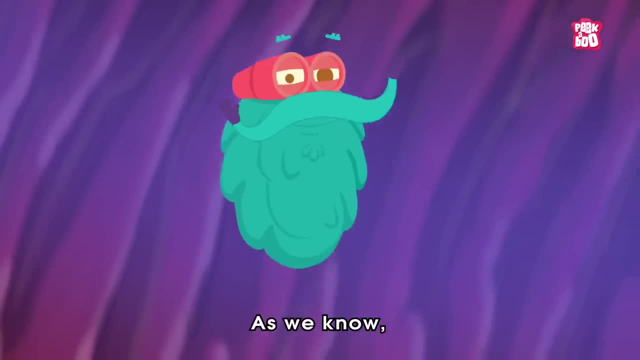 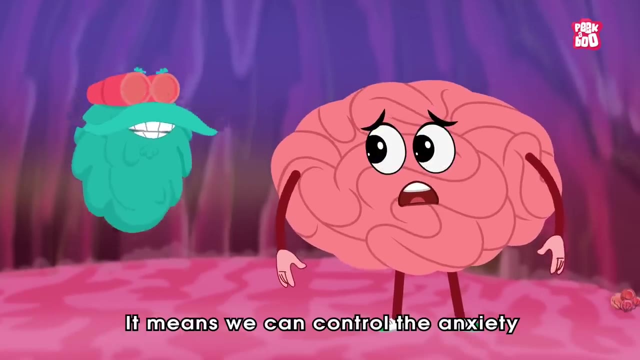 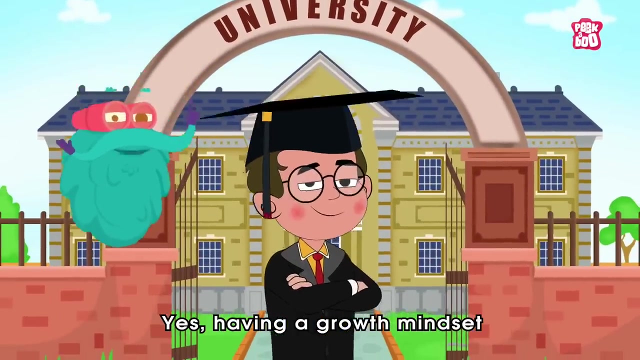 But here's the good news. As we know, math anxiety has more to do with our brains. It means we can control the anxiety by changing our mindset towards math. Yes, having a growth mindset that you can achieve anything can actually help you get better at math. 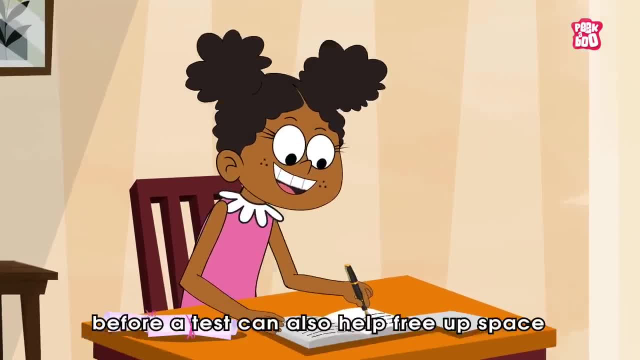 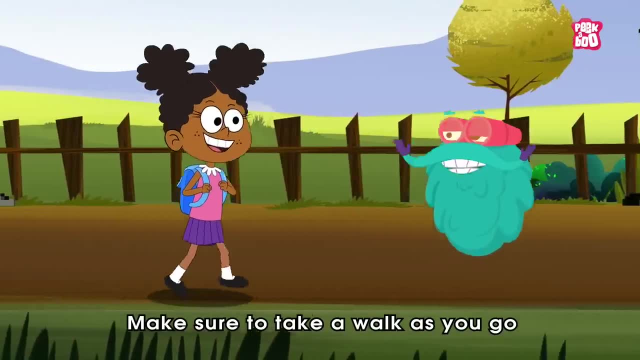 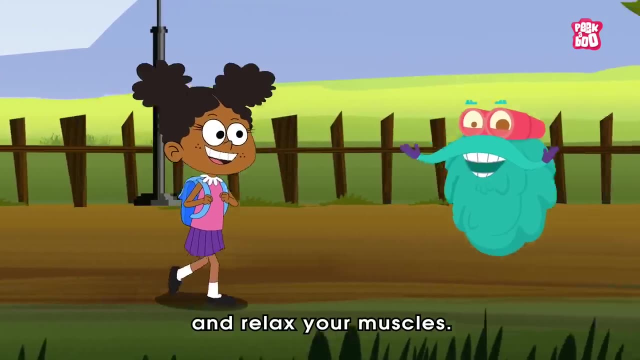 Besides writing down your anxious thoughts before a test can also help free up space in working memory. Make sure to take a walk as you go to attend the test to ease up the tension and relax your muscles, Additionally practicing relaxation techniques such as deep breathing. 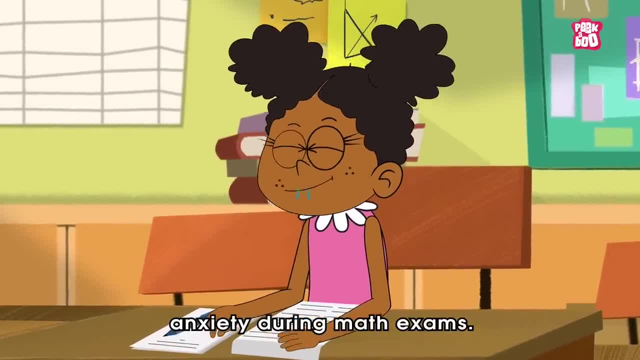 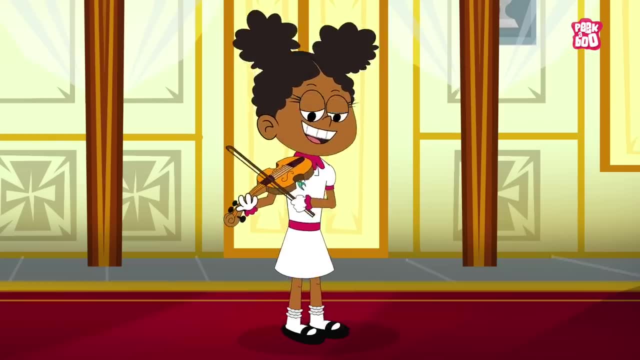 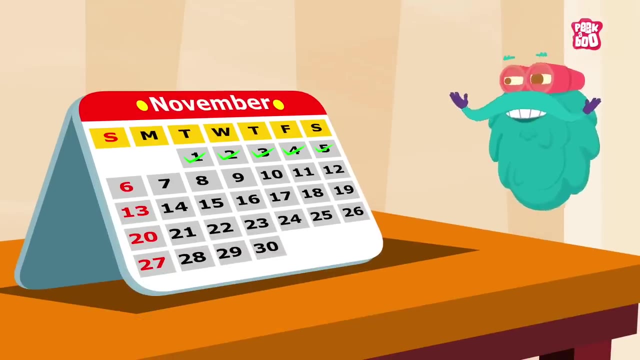 can help reduce anxiety during math exams. And, most importantly, just like playing a sport or a musical instrument, math gets easier with practice. So try to work on math problems every day, even if it's just a few, And remember everyone learns at their own pace. 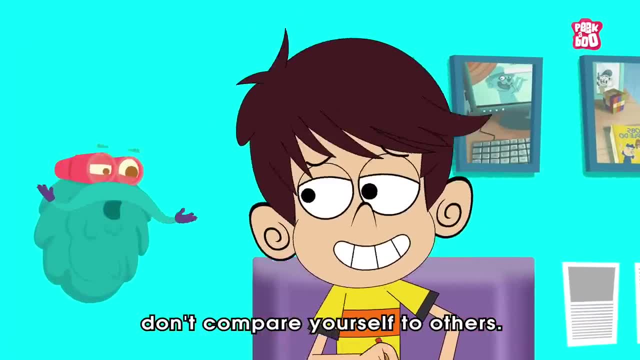 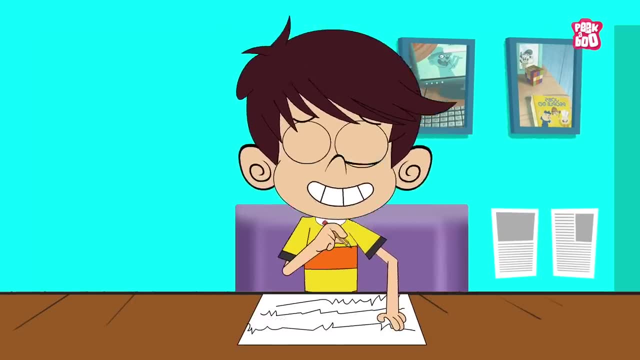 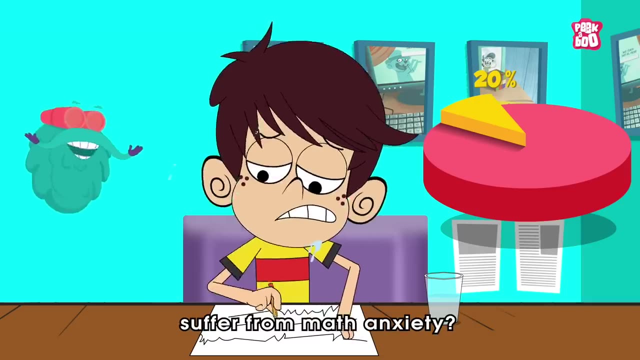 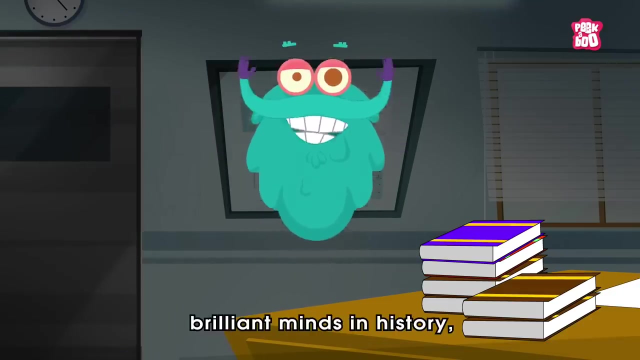 so just have patience and don't compare yourself to others. Just keep going and you'll get better and more confident with time. Trivia Time. Did you know? an estimated 20% of people suffer from math anxiety? But don't worry, even some of the most brilliant minds in history. 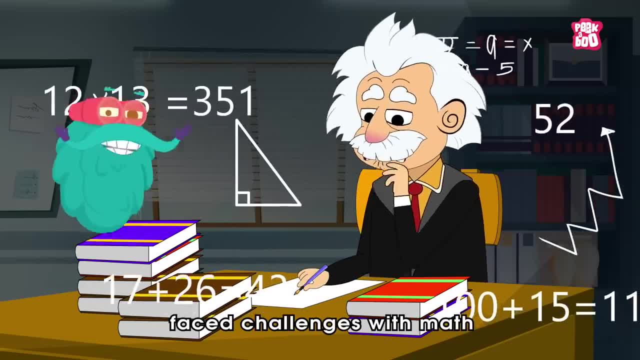 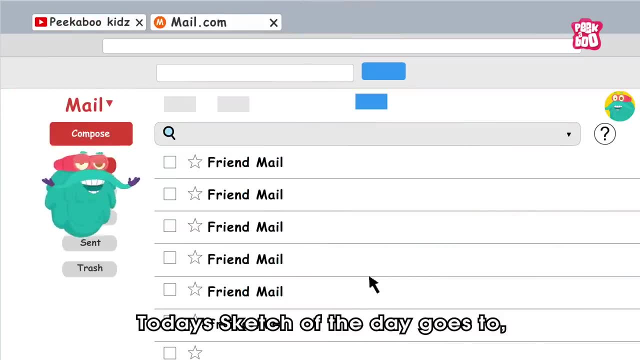 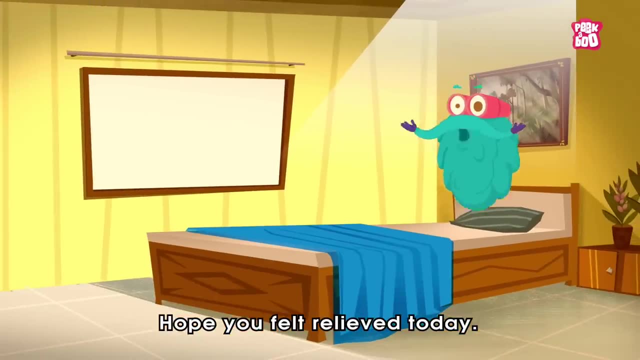 including Albert Einstein, faced challenges with math at some point in their lives. Sketching Time. Today's sketch of the day goes to Lisa Saha. Hope you felt relieved today, Until next time it's me, Dr Binox, zooming out. 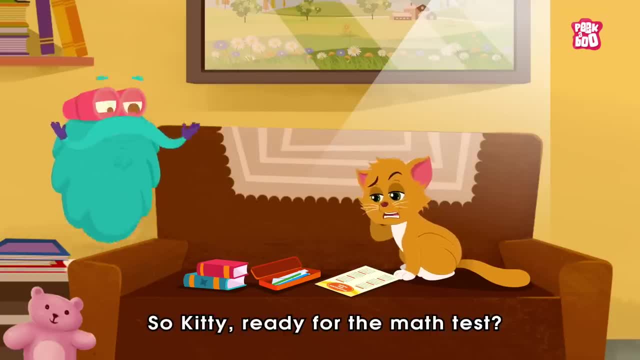 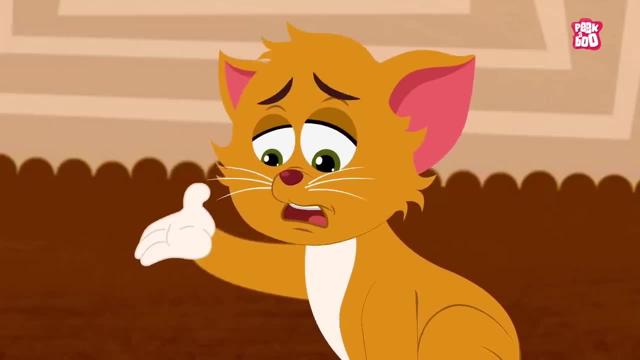 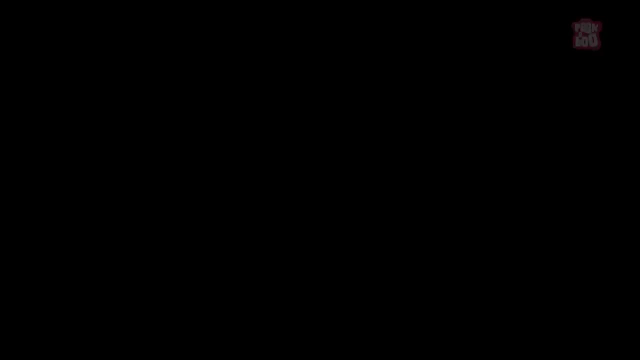